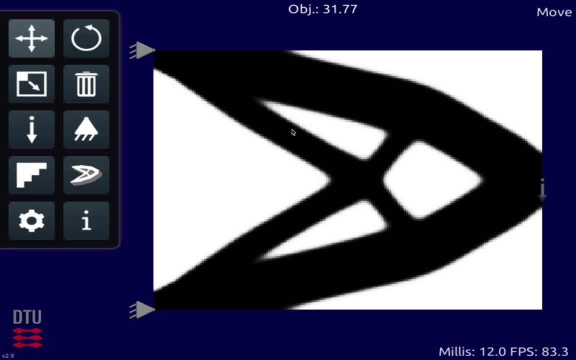 And here we see we have a structure optimized to support a node appearance. So we put a load applied here and this structure is fixed at the top left and the bottom left. Now, if I move the location of the force, the structure would be adapted. 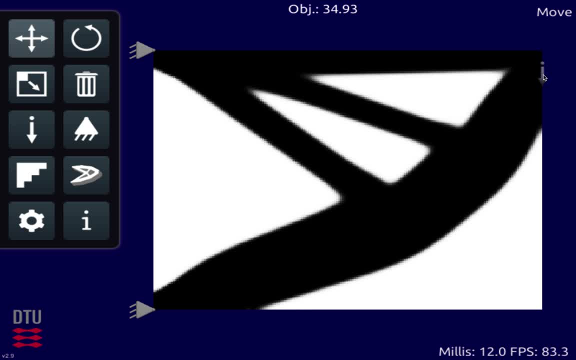 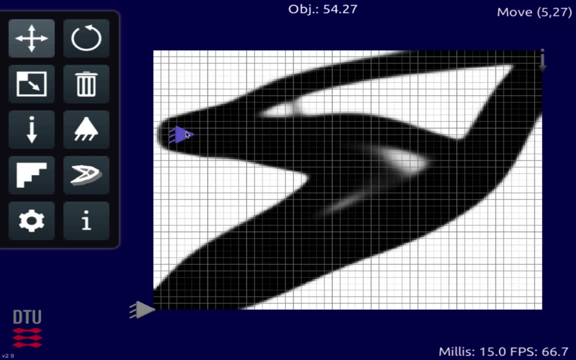 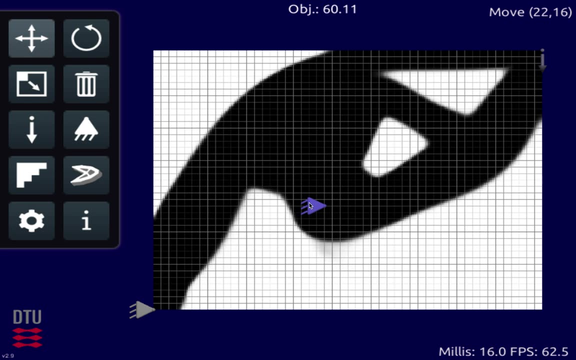 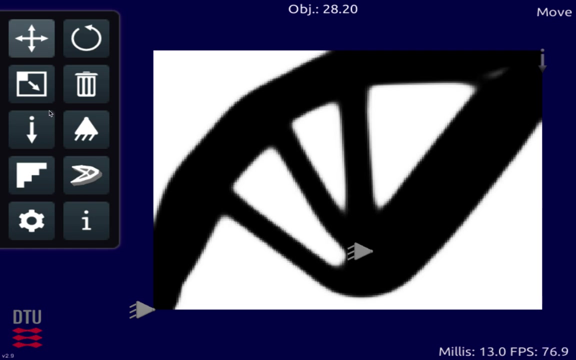 Apparently, the structure is optimal for a particular load case, So we could also move the fixation. If we move it this way, so it automatically adapts. On the left hand side of my screen you see 10 control buttons. Now we would like to design a chair. 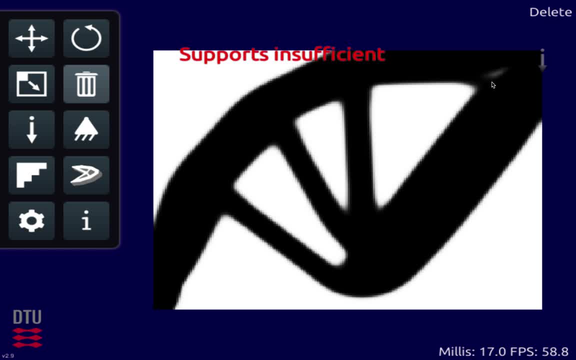 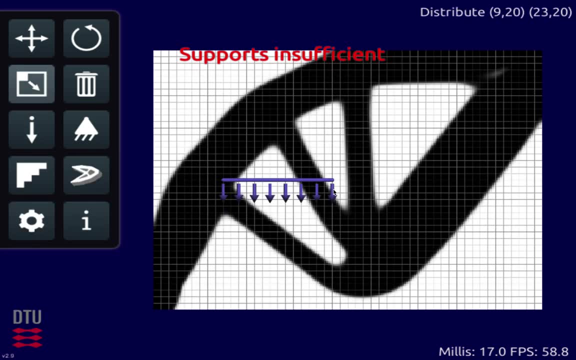 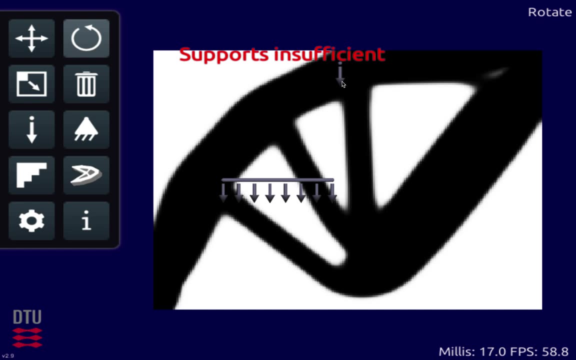 So let me delete this boundary condition. first, We will place a force, We extrude it to indicate the distributed load on the seat, And we place a second load, Rotate it, The back pushing force. Until now, the geometry doesn't change. 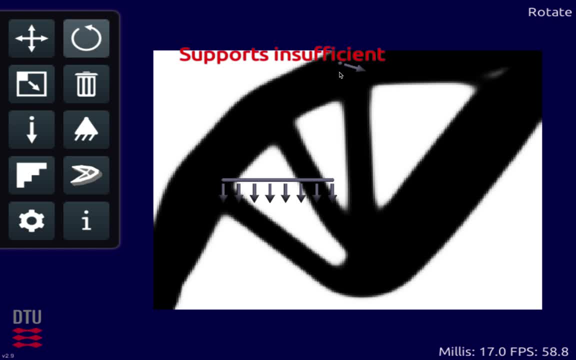 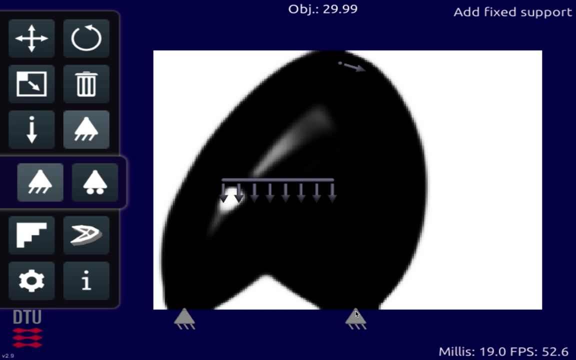 Why is this so? Why it doesn't change? There is a hint: supports insufficient. Think about it. If we place some fixations on the ground, it doesn't change until I place two fixations. Then the geometry starts to evolve. 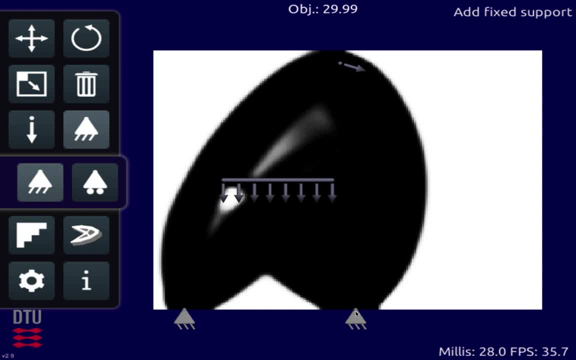 And this has to deal with the So in 2D. if we have a structure, it has three degrees of freedom. It can move in X and Y direction, It can rotate, So it has three degrees of freedom. And if we don't have more than three fixations, 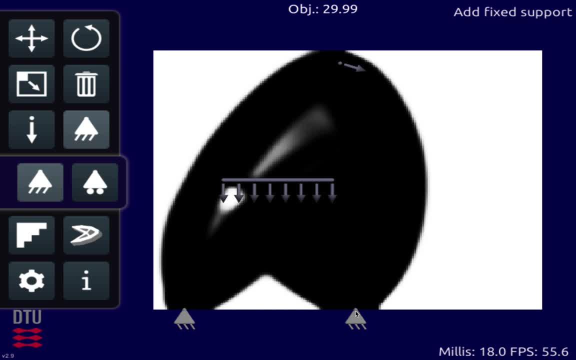 or more than three degrees of freedom fixed. that means the geometry could move almost randomly. It is mechanically indeterminate, But as long as we have two fixations, each of the fixations controls X and Y direction. So we have four degrees of freedom fixed. 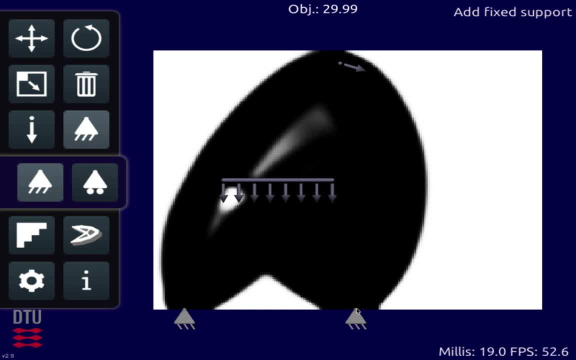 Now we could. The problem is determinate and the geometry starts to evolve. Now we have optimized geometry for this boundary condition. It doesn't really satisfy our expectation. We are looking for a chair, which means this part: the person should accommodate the person. 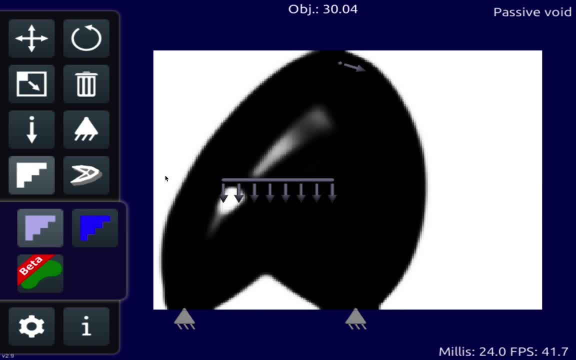 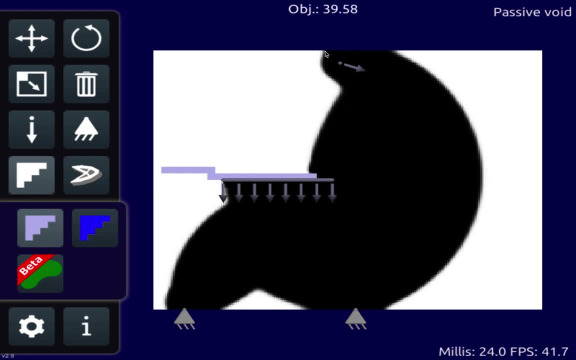 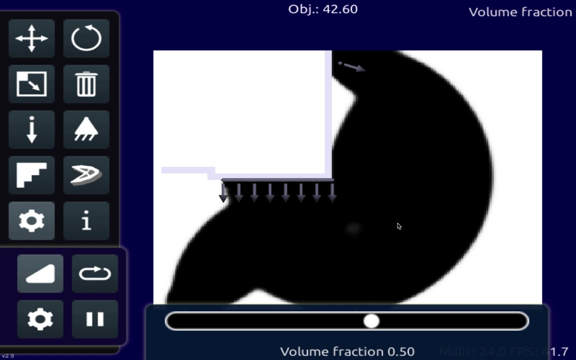 What we could do here is we tell the optimization to not place material in this part, which we call passive region, And we extrude, exclude material from this part. Looks reasonable, now Looks a bit bulky, So we could tune the volume ratio. 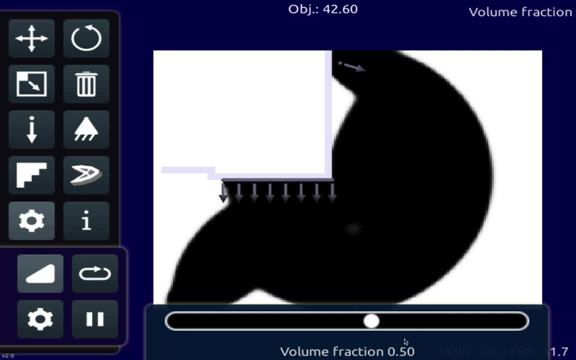 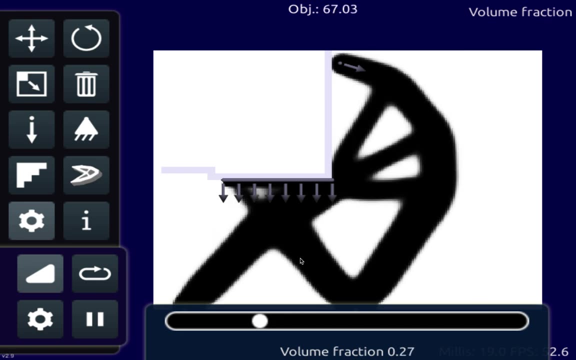 Here it says 50%, which means the design domain. 50% of pixels are occupied by material, So we could make it smaller. Let's say we make it 27. And it becomes: The volume becomes smaller, It becomes more porous. 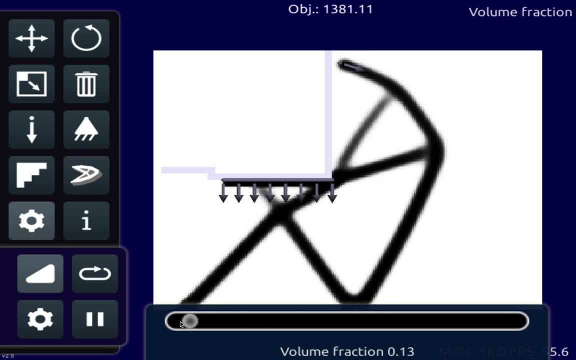 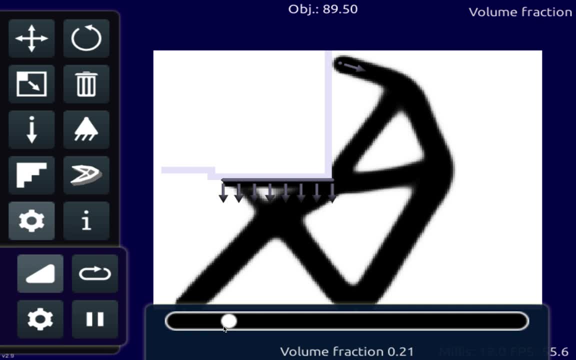 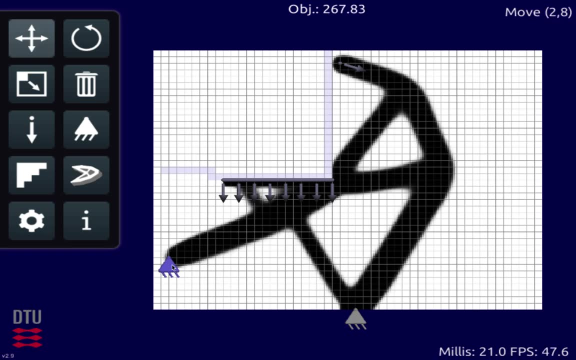 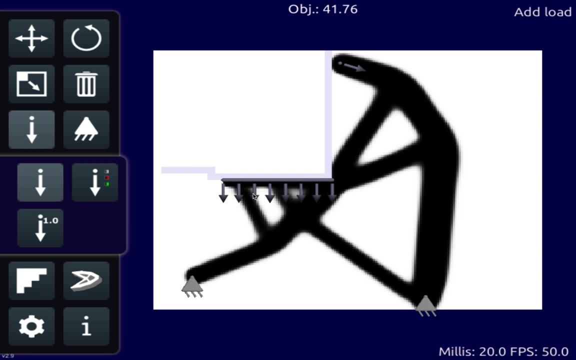 We could make it even smaller. So it is always the geometry that's under this volume fraction to maximize the stiffness. You could further customize it. For instance, you could move the location of the fixation. You could also, You could also tune the relative force. 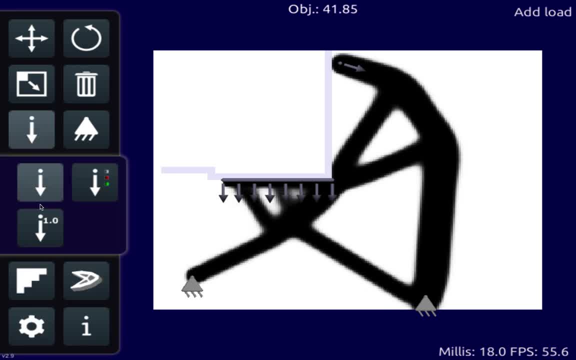 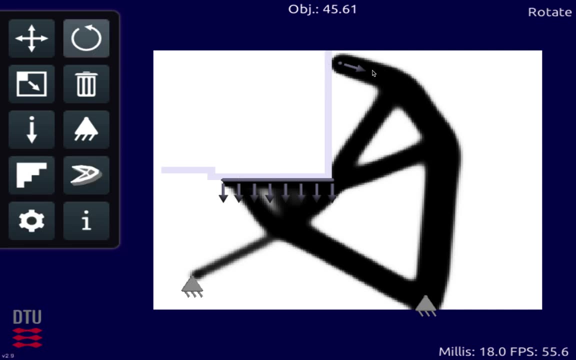 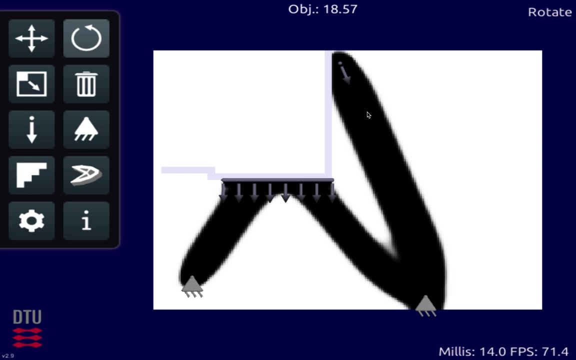 Oh sorry, It should be this one. So make the force larger. Now it's. Oh sorry, Now it should be making the force larger And you could also rotate the force. So as long as the boundary conditions changed, the best structure to support this boundary condition. 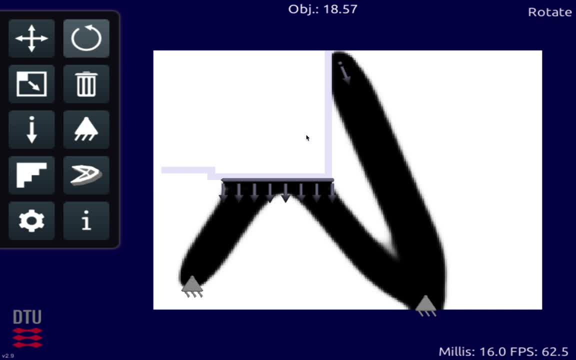 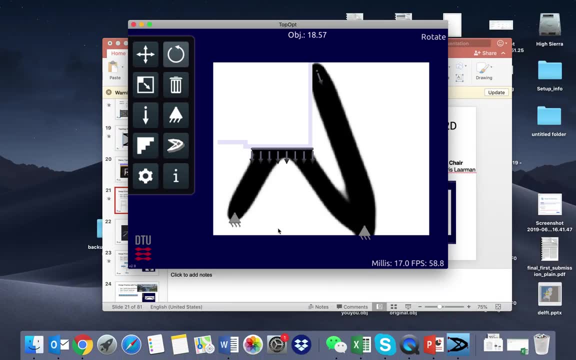 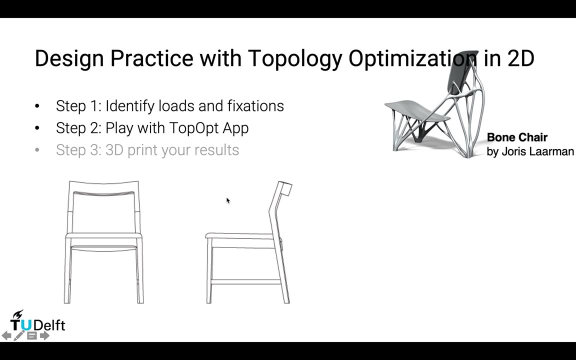 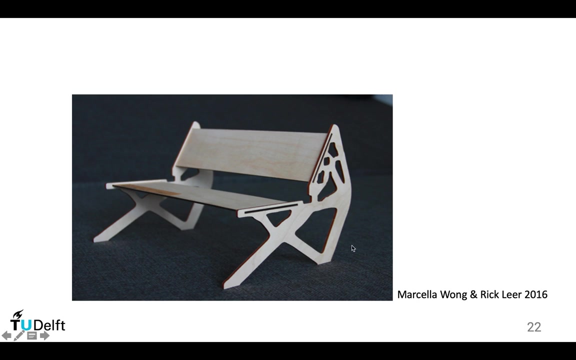 is automatically adapted in almost real time in 2D. All right, And now let's move back to our slides. So we have prescribed the boundary condition and we find a very elegant structure like this, And this is a group of students did in 2016.. 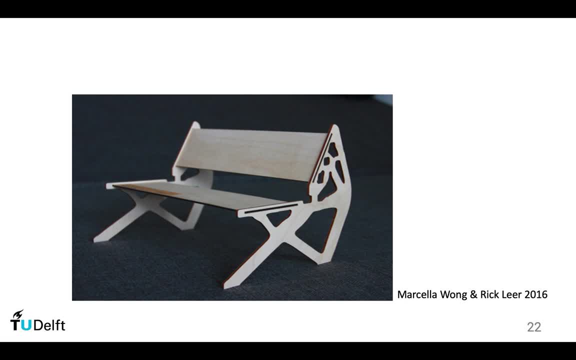 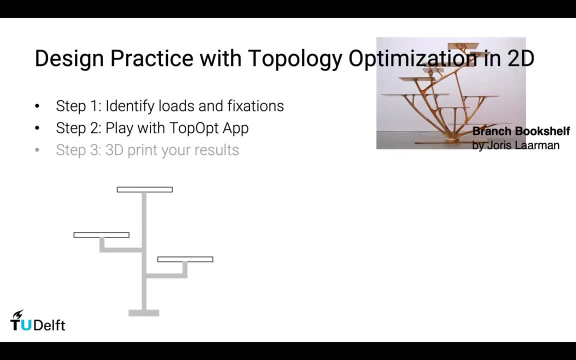 So they used this app to design these two sides of a bench, And this one was fabricated by laser cutting. Looks very interesting. In the same principle, you could apply it to design this multi-layer table or this multi-layer bookshelf. So the principle, or the steps are: